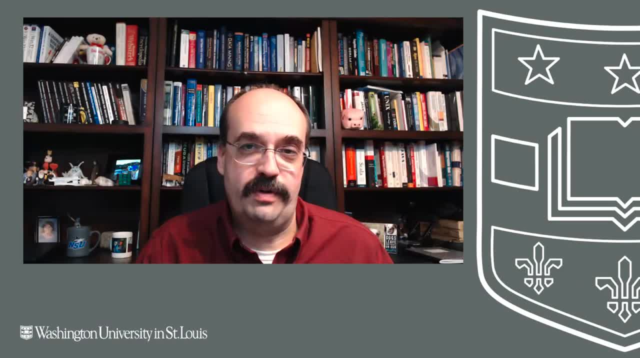 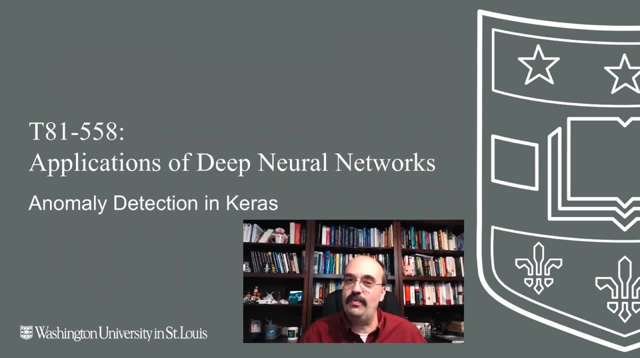 Hi, this is Jeff Heaton. Welcome to Applications of Deep Neural Networks with Washington University. In this video we're going to look at anomaly detection. How can you detect something that is not the way it should be? This has great application in computer security, but in other fields as well. We'll have a look at that in this video. 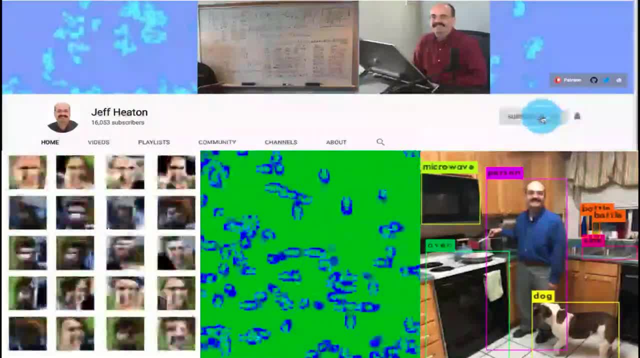 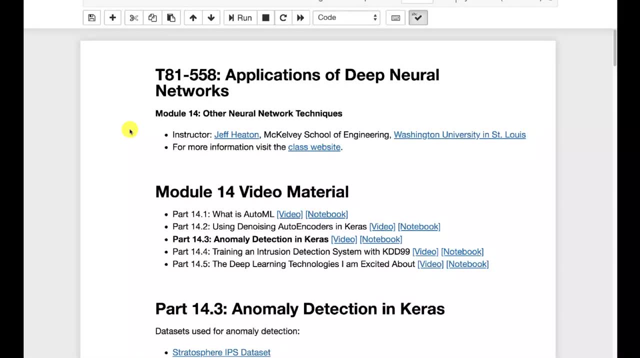 For the latest on my AI course and projects, click subscribe and the bell next to it to be notified of every new video. So now let's look at a use of autoencoders. We're going to see how an autoencoder can be applied to anomaly detection. 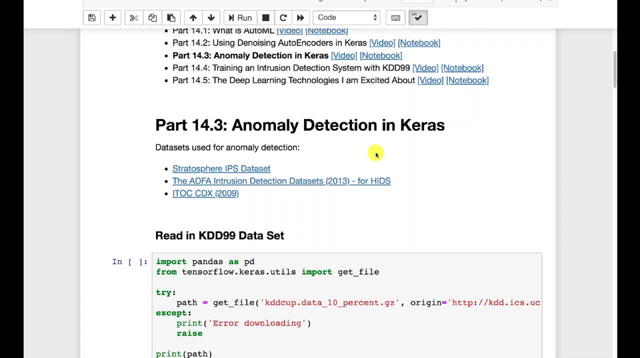 I have a link to a couple of other tutorials on the internet that talk about various ways to do anomaly detection in Keras. Some of these might be useful to you. The approach that I'm using here is using an autoencoder and looking at the error of the autoencoder to determine if the data are unusual compared to. 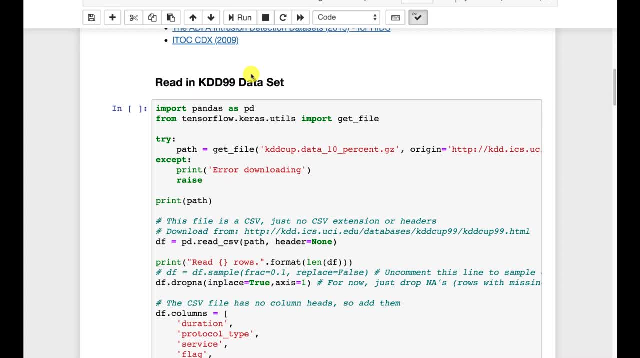 the previous one. We're going to make use of something called the KDD99 dataset. We'll use this in two parts of this course. We'll use it to create an intrusion detection system in the next part. This is an older dataset- At 2019, this is now going on 20 years old. 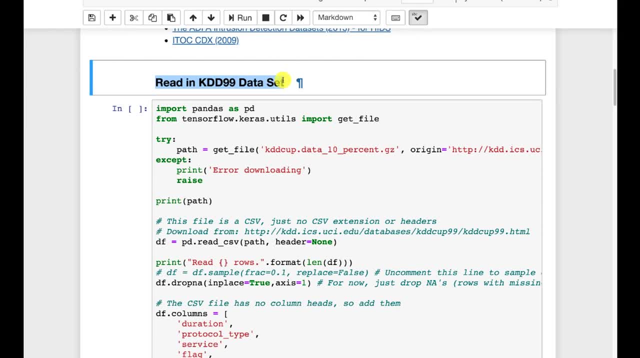 So this is? this is an older security dataset. It's got enough columns and whatnot that it is useful. I don't know that. I would base anything on current research, meaning trials. I'm not trying to create systems that detect current intrusion detections or current anomaly detection based on 20-year-old data. 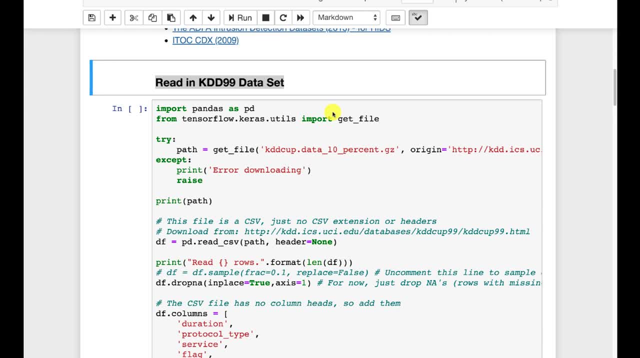 But it is a good sort of hello world for security and it's non-trivial. It's a decent amount. It's not big data by any stretch of the imagination, but it's useful. So we'll see it here. It's good for examples. I wouldn't use it for current research. 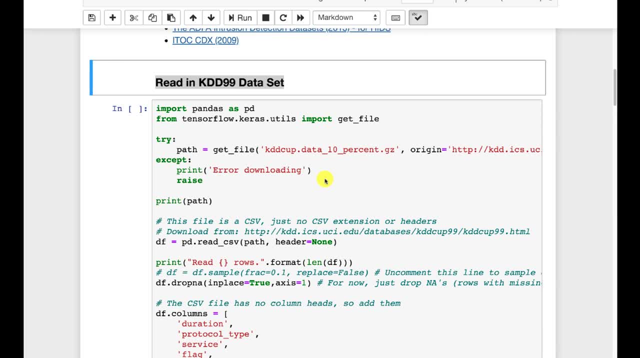 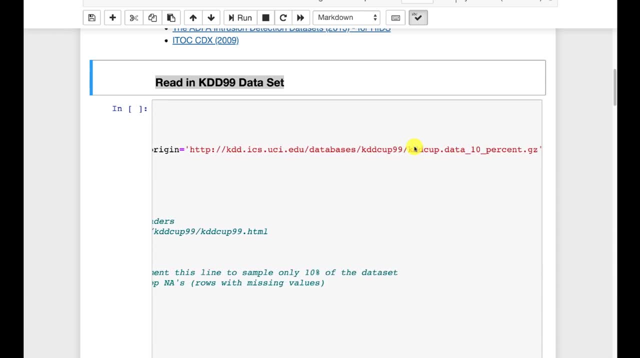 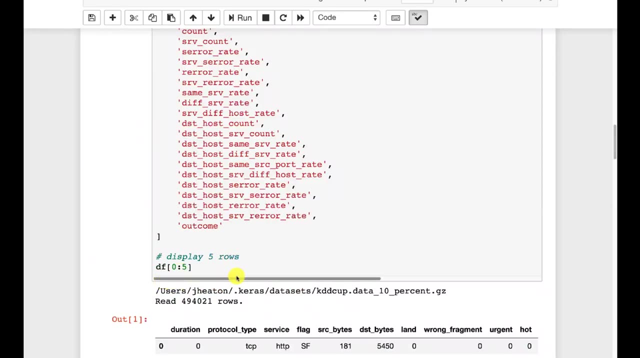 That being said, I see papers published with it frequently, but of varying quality. I don't include it with the GitHub repository because it's it's decently large, But this command here will allow you to download it. I'll go ahead and run this. It lets you know where you downloaded it to. 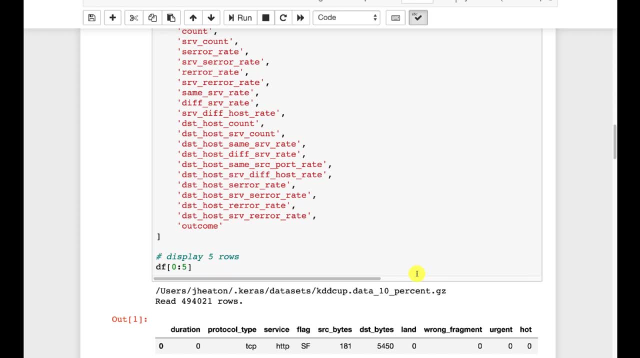 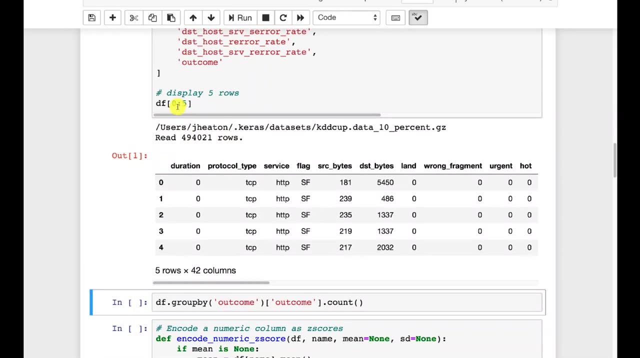 If you're using Colab, you may need to put it on your G drive somewhere. I'll try to put specific instructions for Colab in here. So now we've got the data and I displayed the first five rows, You can see what this looks like. This is network type data. 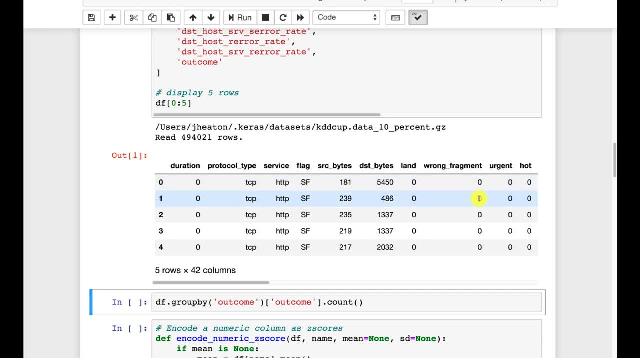 This was created In a simulated environment for a competition KDD kind of an early Kaggle, and doesn't show all the data. There's quite a quite a bit of it, But what I am going to do is let's take this data and group it by the outcome. 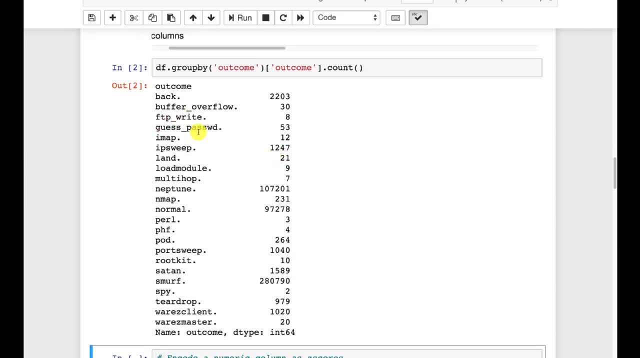 So these are the outcomes: Buffer overflow, FTP write, guest password. Those are all different types of attacks that were simulated in this. Some of these are still attack types today. Some of these are probably pretty uncommon 20 years later, so definitely be be aware of that. 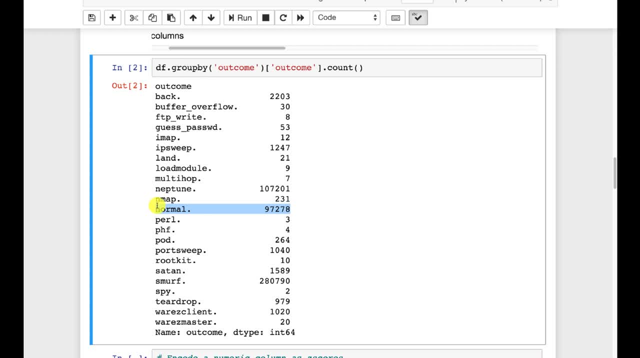 Normal is one we're particularly interested in because that means nothing is happening. So we're going to train it that the normal are well normal and the others are the anomalies. So we're going to train a neural network to detect things that are not like normal. 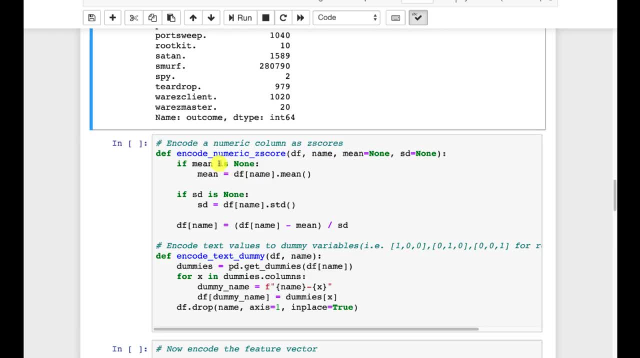 We're going to do this completely with a autoencoder. I create two functions to help us pre-process this: one that encodes the z-scores and one that encodes dummy variables, And this is my pre-processing for it. You can see there's a lot of columns here. 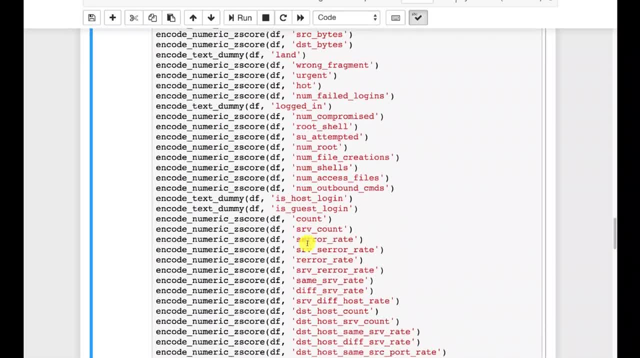 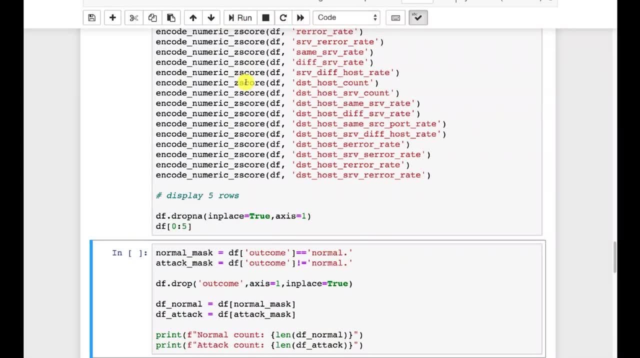 And I'm encoding basically in z-scores and dummies. Those are the only two transformation types that I'm doing, So I'm keeping things relatively simple And we drop any NA's rows that have NA's- There's not really that many. 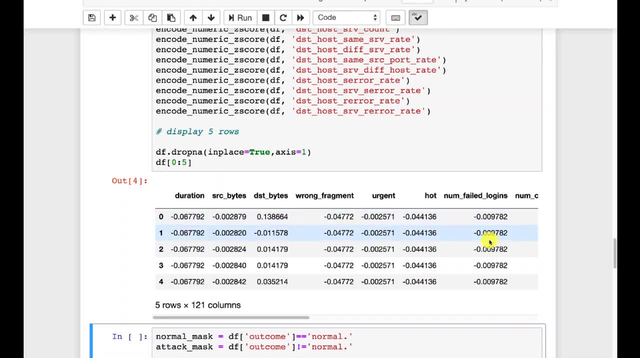 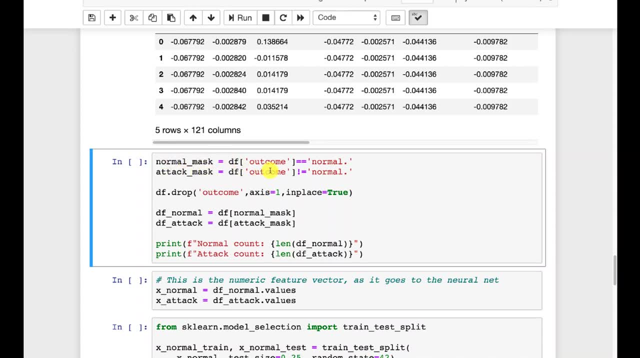 And you can see the rows. here You can clearly see the effects of the z-scores. Now what we're going to do is create a mask that has the normal and the attacks. That way, we're able to segregate this data. We're going to drop the outcome because we're not really training on the outcome. 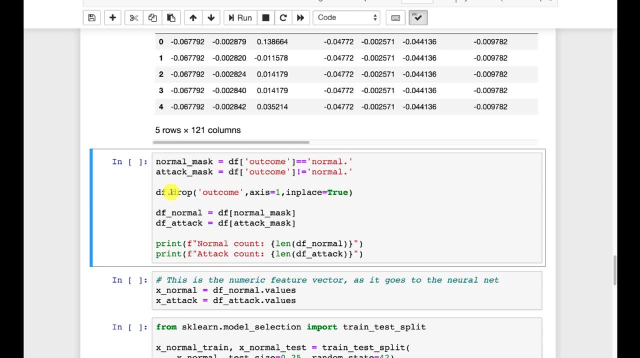 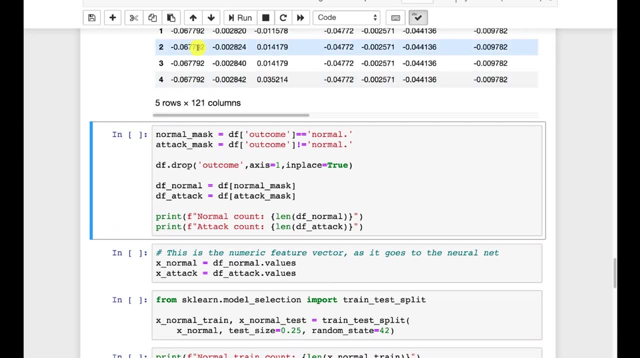 That's essentially the target. Really, this is unsupervised learning. once you get it separated into these two groups, such as the nature of autoencoders, We'll go ahead and run that And you can see. the normal count is about 97k. 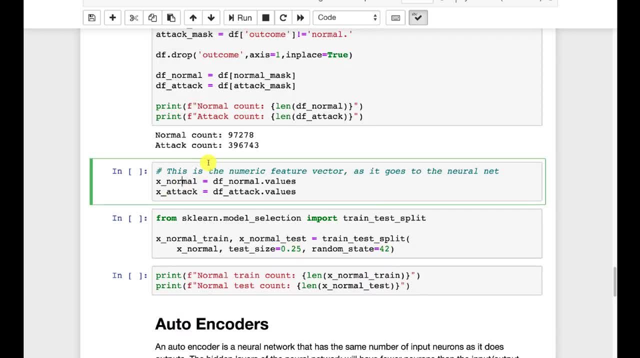 Attacks are much more common in this dataset. We separate it out so that we have the x for the attack and the x for normal, And then we're going to break this into a table, Into a train test split. We're breaking normal up because we're going to use normal to evaluate it. 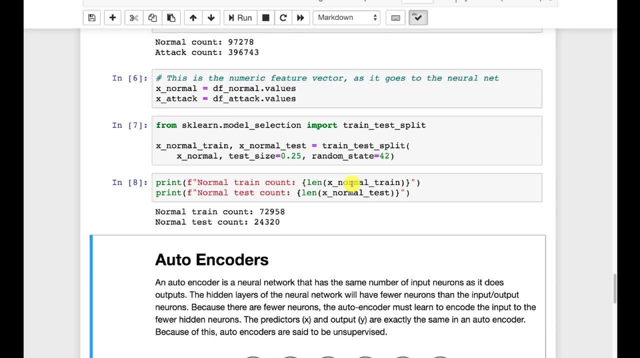 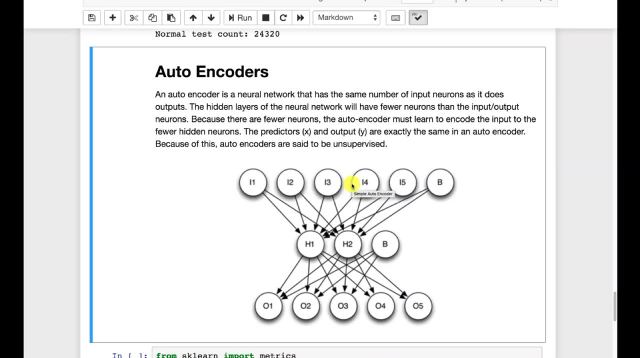 We're going to see if the normal looks like normal data to it, Non-anomaly. Now we're going to use an autoencoder for this, And we've talked about autoencoders before, but just so these videos somewhat stand alone, just to give you a quick overview of this. 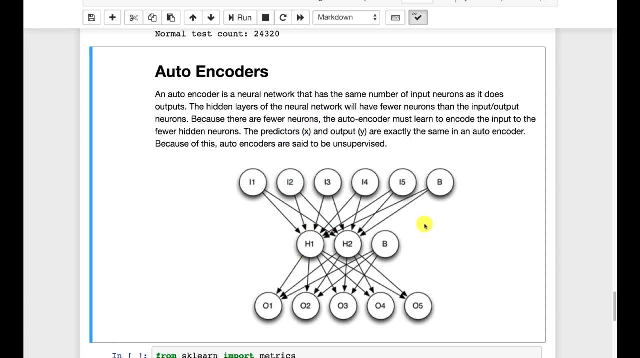 An autoencoder is essentially a neural network that has sort of a skinny hidden layer structure. The idea is A number of inputs. Now you're going to have all the KDD 99 inputs. for this particular one You do have the bias neurons, like you do in most networks, and you have an output count. 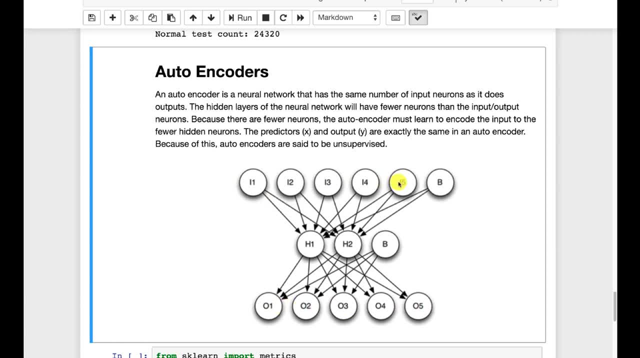 equal to the input count, And what we're going to do is basically train the autoencoder so that it is able to produce the same input as output. Now, that seems useless, but that is teaching it essentially to do feature reduction and simplification. 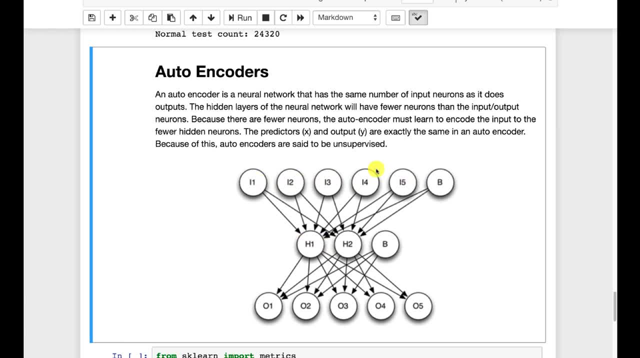 So it teaches it to take all of these inputs. These five inputs are hundred, as we will have probably with KDD 99, and represent them as just the two numbers being output to the hidden one and hidden two. Now, all the weights leading into here are the encoding weights and these are the decoding. 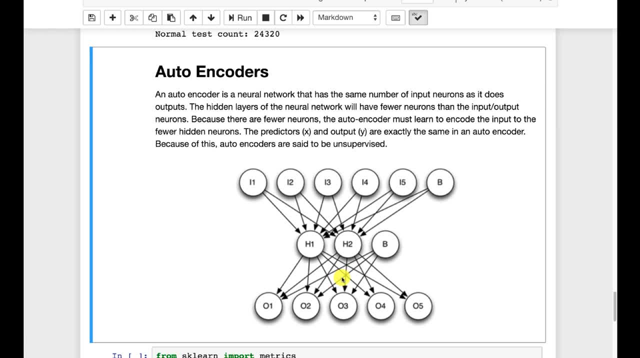 weights. So those are what it learns for how to decompress it. Here we're going to build our autoencoder. We are going to have a little more complicated of an autoencoder. They're going to have a little more complicated of an autoencoder. 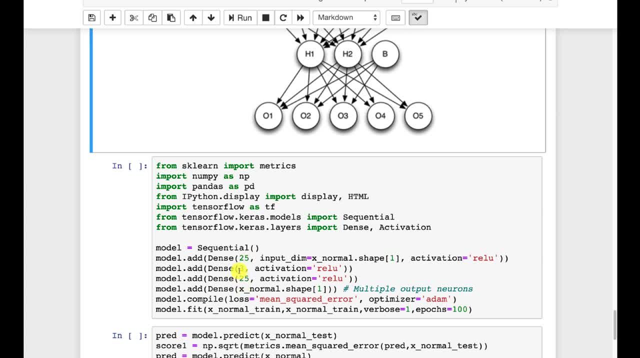 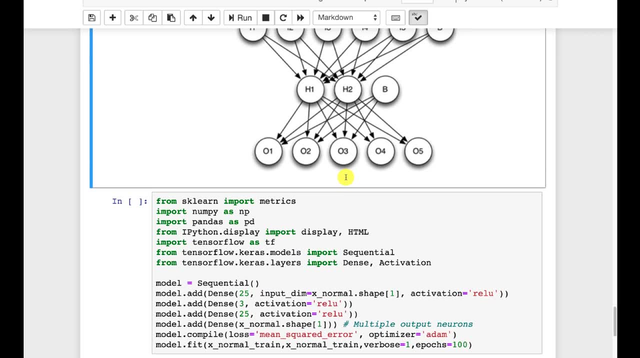 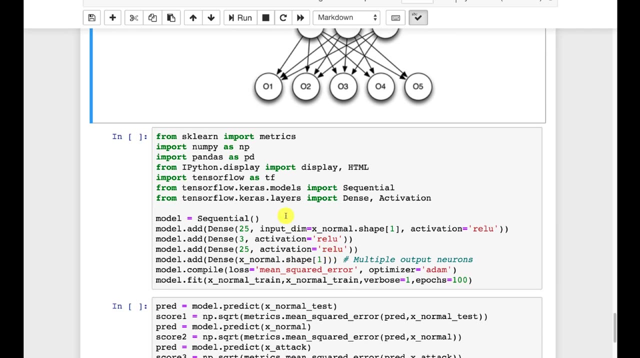 So we're going to have essentially 25,, 25,, 3.. We still have this very thinning area, but we have a little bit of sort of an hourglass. So it's almost like we have three hidden layers here to actually give us our compression capabilities. 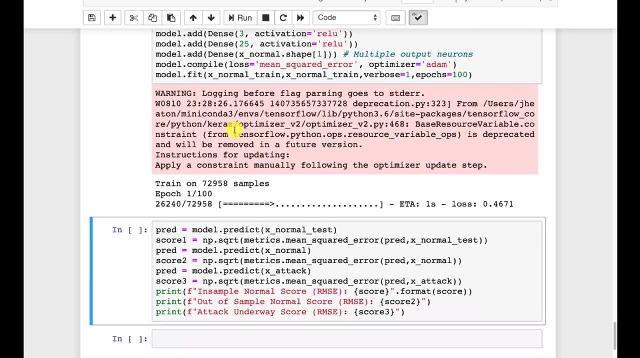 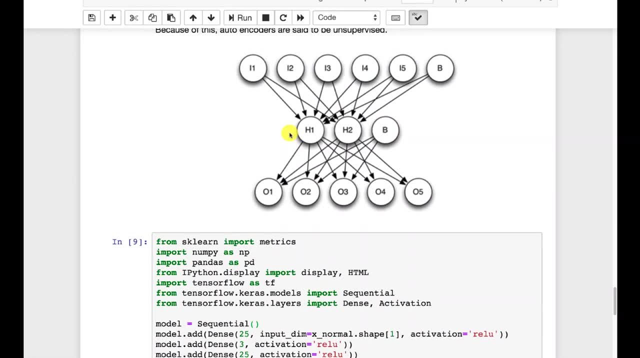 So I'm going to go ahead and run this. It will actually fit it. So it's going to take it a little bit to fit this neural network. I will fast forward this part. Okay, It's trained. Just to explain. Let's get into the theory of what's going on here. 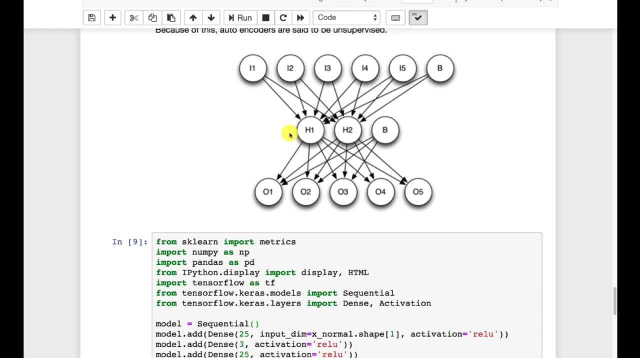 We train this just on the normal data and it is being trained unsupervised, So we're not even giving it the outcomes. There'd be no point to give it the outcomes because they're all normal, So the outcome would be the same. 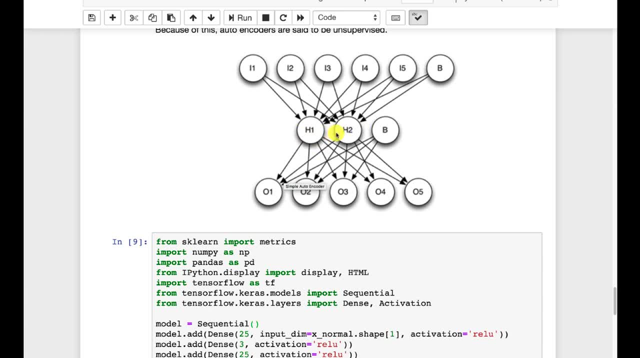 Since it's learning to compress to reduce the dimensions. the way that dimension reduction or compression in general works is by using patterns to represent common portions of the data. It's simplifying it. That will only work on cases where the data coming in is pretty similar to that. 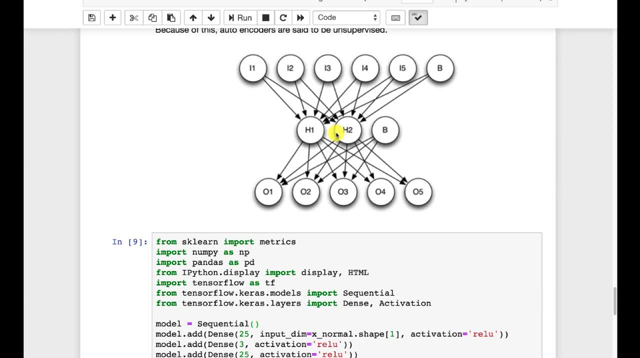 Now I'll give you a perfect example of a unintended anomaly detector. Now cell phones are a lot better about this, but earlier cell phones the way that they would compress is they knew a lot about the human voice that would normally go through there. 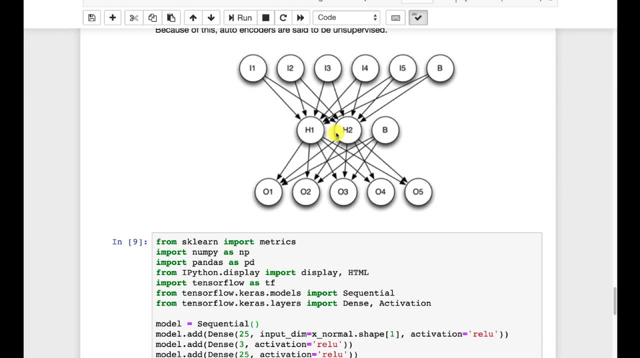 So they use the ranges that the human voice was normally in. They only compressed it and degraded quality in such a way so that it would not be annoying for human voices. You'd still recognize the voice. You would still be able to understand it. 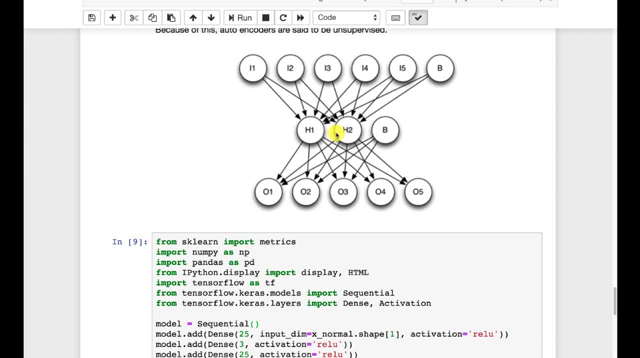 However, if you tried to play music through a cell phone or other other tones that the compression algorithms simply were not designed for, they would not be reproduced as well. There would be static and other distortions in them because those different tones other 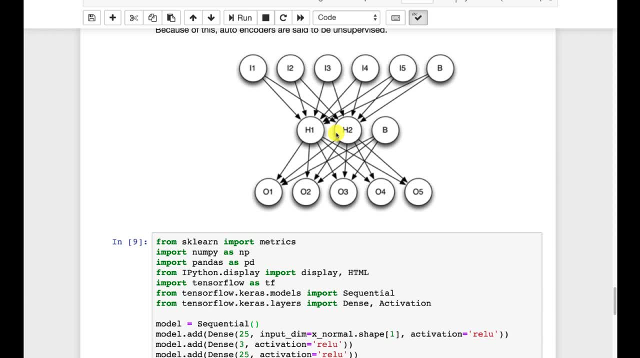 than what the compression algorithms were built for Are different. They're anomalies and the cell phone detected the anomaly, not what it's designed for. It's just an example, but it detected the anomaly by distorting it. That's what we're going to see here. 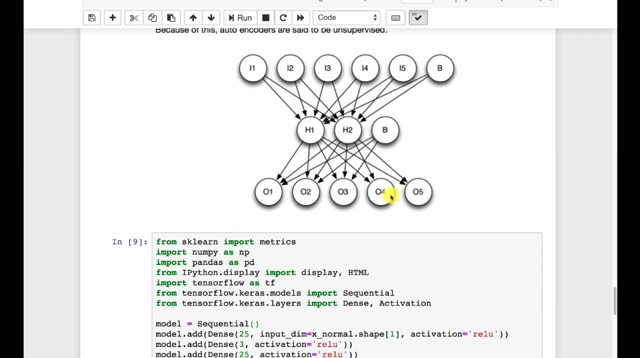 We'll put data into the input and look at how similar the data is in the output to the input, because the auto encoder is meant to be a straight pass through, but it compresses in the process, So it compresses and then expands and we want to make sure that we're not seeing too much. 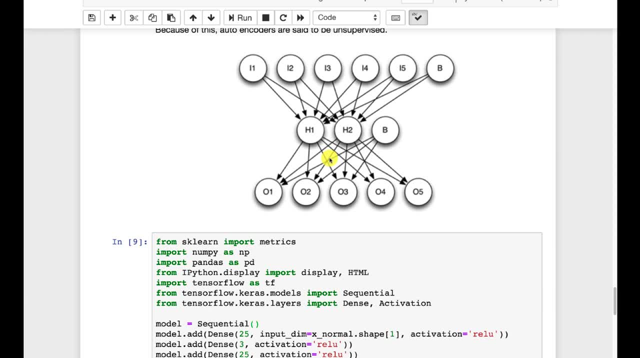 distortion. We want to make sure that we're not seeing too much distortion in that process because if we are, then the data coming in are probably different than the data that this was originally trained for. Now, we saw earlier in this course that you could use chaos statistics and other things. 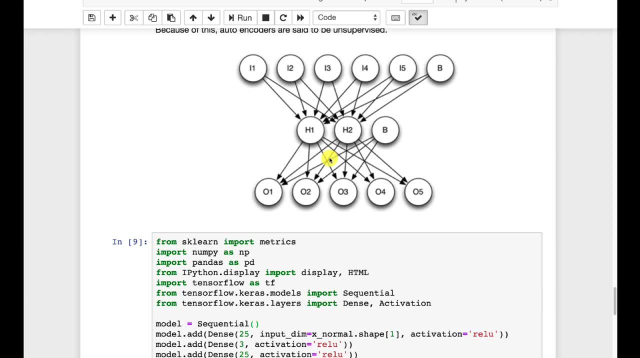 to determine if your data have changed to the point that your neural network might need to be retrained. This is another great way to do this: Anomaly detection and detecting if your data is sufficiently like the training data to know when to update your neural network.